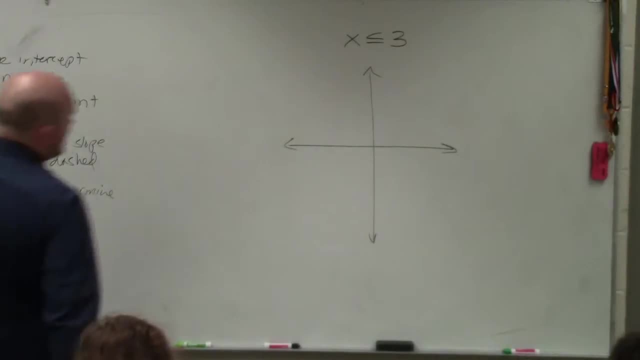 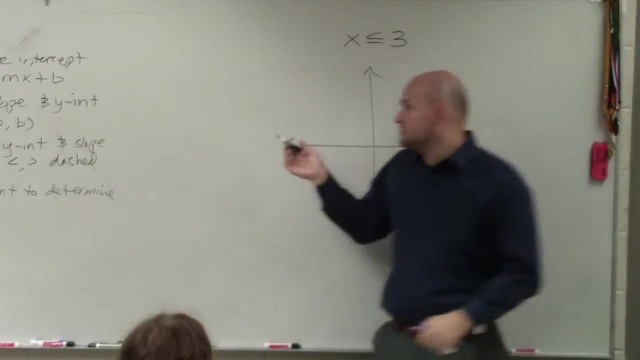 OK, So let's go ahead and get into this. So, ladies and gentlemen, if we were going to graph this, the best thing I can tell you guys, when graphing x is less than or equal to 3, is just to think about how would you graph. 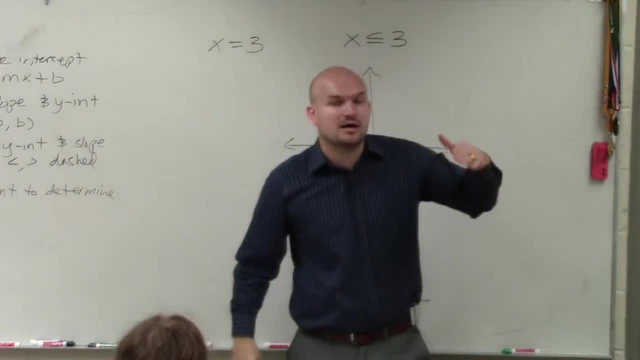 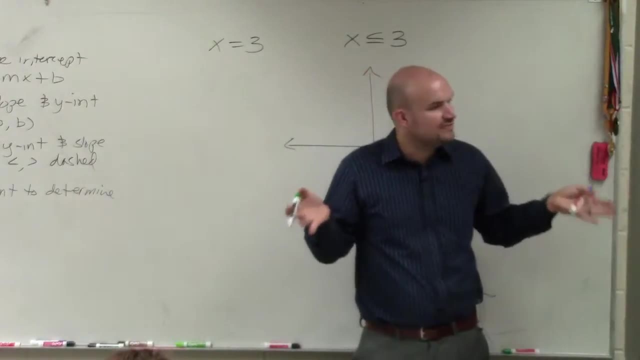 the line x is equal to 3.. And if you guys remember, in our focus lesson two class periods ago, we talked about how to graph x equal to 3.. Yeah, it creates just a vertical line. Use a table of values if you need to. 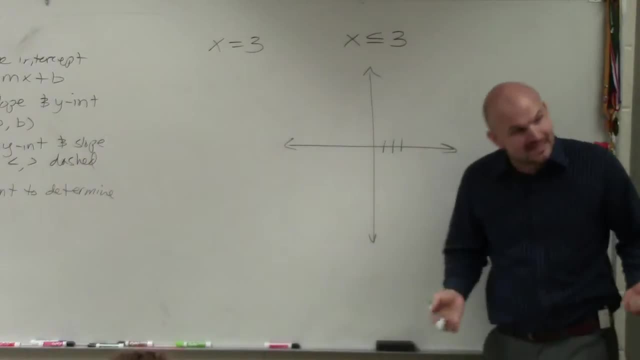 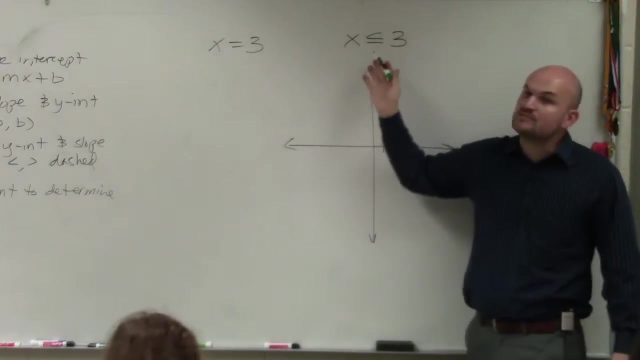 Basically, we know that x is equal to 3, and it's always equal to 3.. So, no matter what the values of y, x is always going to equal 3.. Now, since we have a less than or equal to, 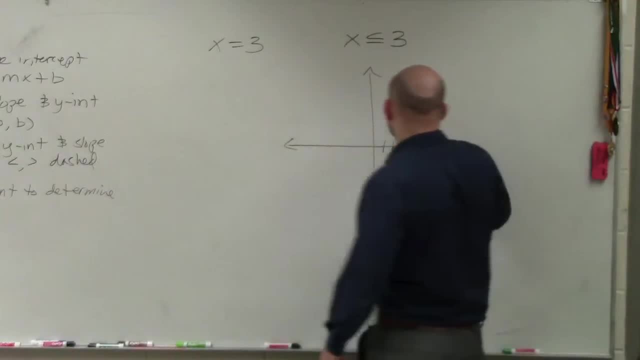 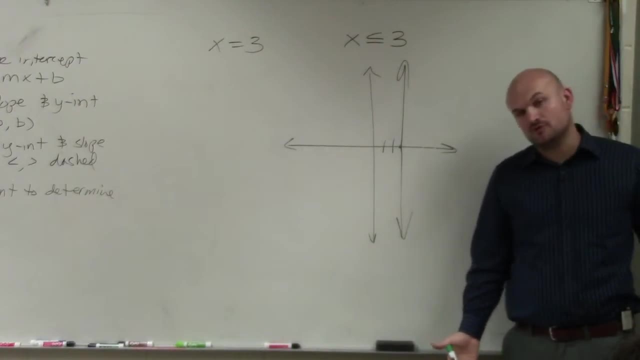 we know that we're going to have a solid line. Our points on this line are going to be a part of the solution. Now all we simply need to do is twofold. You can think. you can kind of go back to what we talked about. 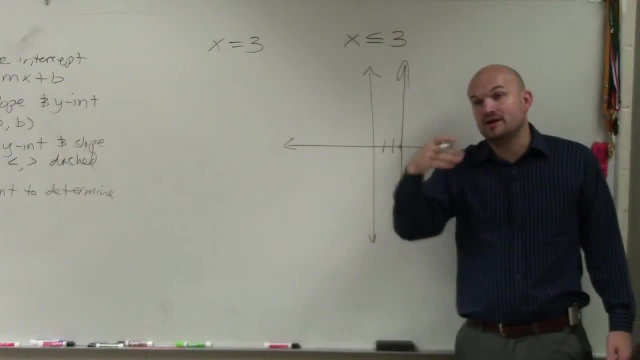 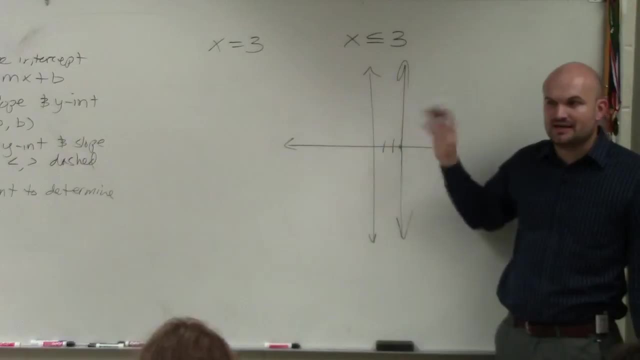 We can kind of go back and talk about the one variable number line And just think about it. Now again, we're talking about linear inequalities here. So that's why I knew to graph it on x and y-axis. And you will be told to graph on x and y rather than just 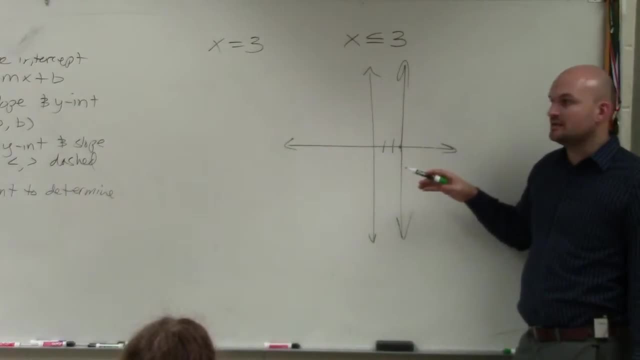 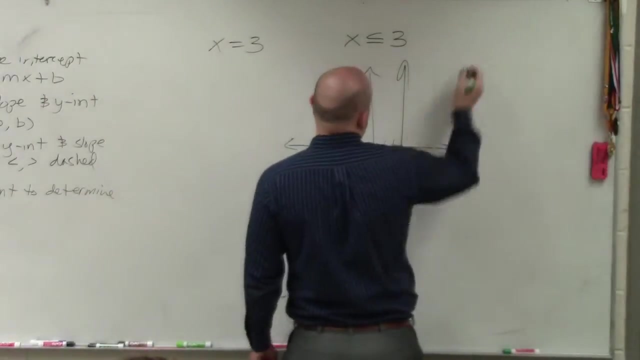 an x-axis, But what are all the values that are less than or equal to x? Are they to the left or to the right Left? So you could do a test point. if you wanted to, You could still do. 0 is less than or equal to 3.. 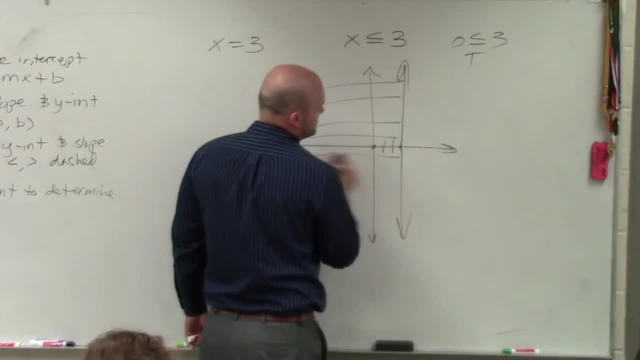 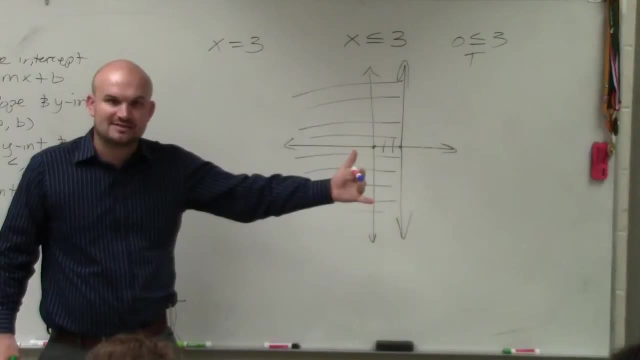 That's true, But then you just shade to left. So just remember, guys, when you have x is less than greater than equal to whatever, that creates a vertical line, It's a vertical line at the value of x. 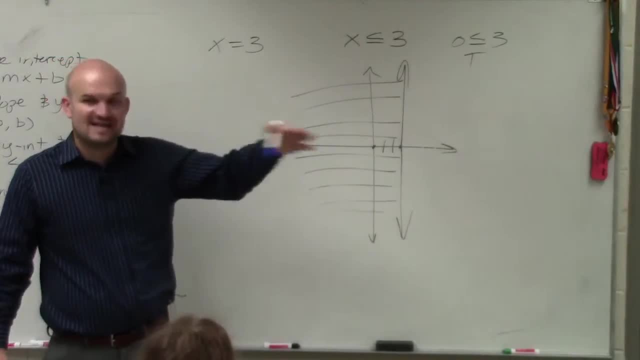 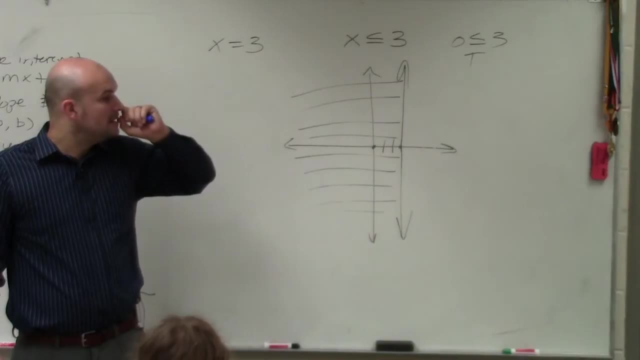 If you had y less than greater than equal to whatever, that creates a horizontal at the y value. Yes, Are we going to have to do stuff like that on the test? Not this test, Maybe on the other test? No, actually this is. 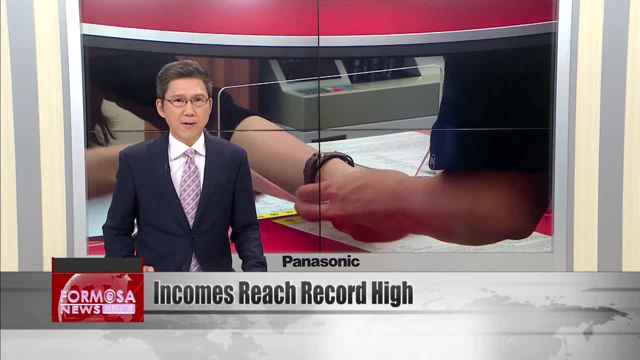 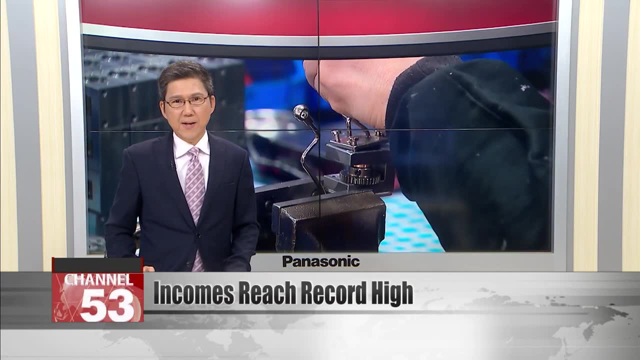 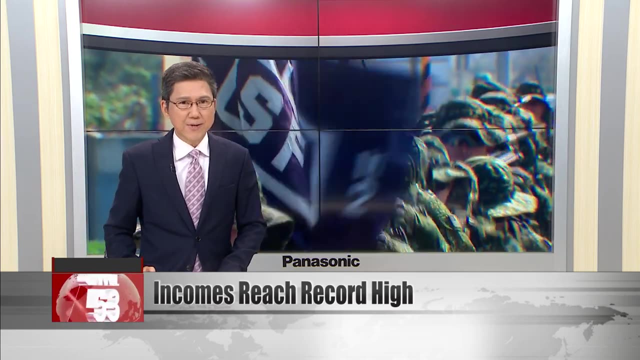 A new government survey has shed light on incomes in Taiwan and revealed a new record average for annual income last year: 700,000 NT. That rise in average income holds across the board for different age groups. Experts say steady increases to the basic income rate have been a driver of.